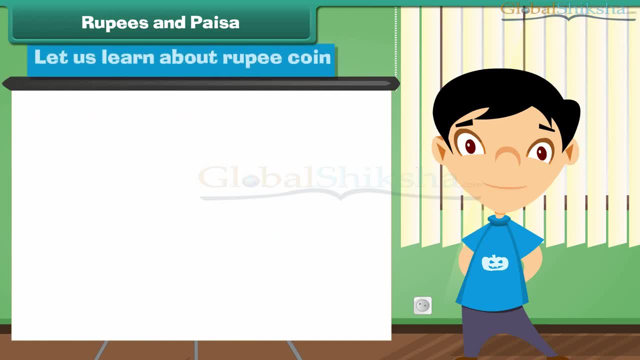 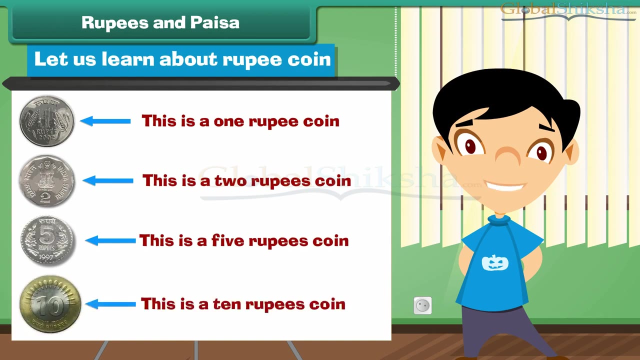 this is 50 passive collection. let us learn about troopee coin. this is a one rupee coin. this is a two rupees coin. this is a five rupees call-in. this is a tender peace call. it's. learn about rupees. note this is and one dripping. 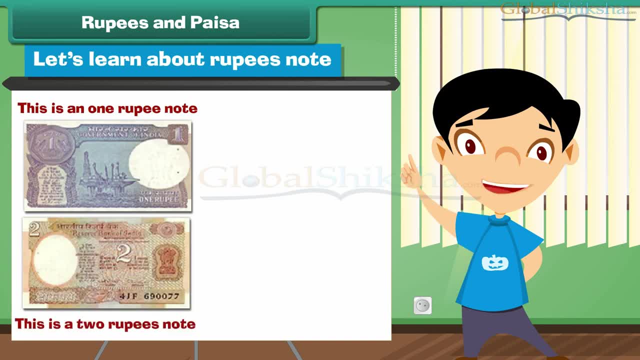 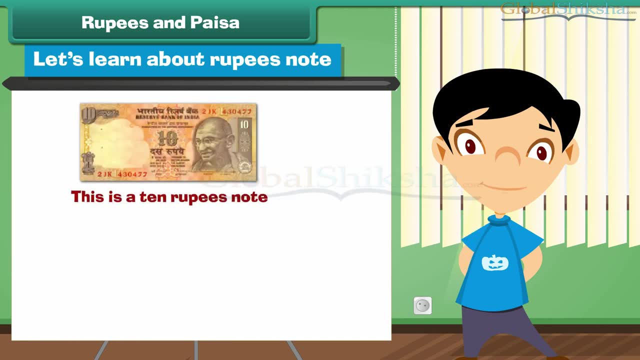 note. this is a fan rupees note. this is a five rupees god. This is a Rs 5 note. This is a Rs 10 note. This is a Rs 20 note. This is a Rs 50 note. 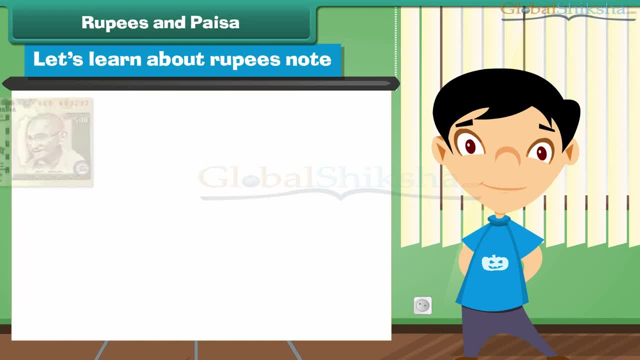 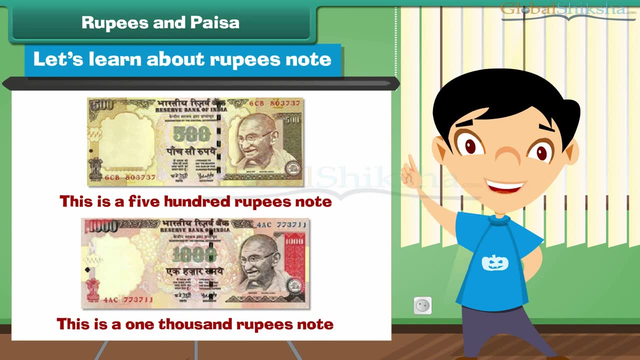 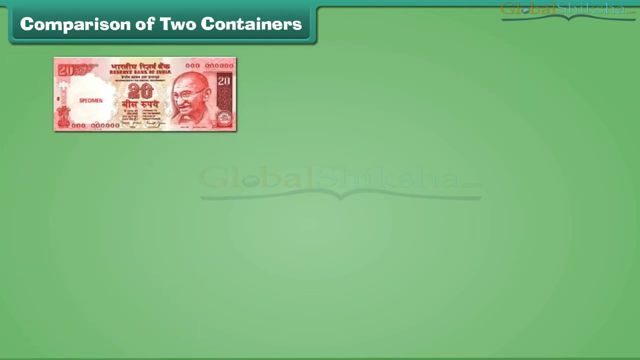 This is a Rs 100 note, This is a Rs 500 note And this is a Rs 1,000 note. This is a Rs 20 note. A Rs 20 note is equal to the sum of 4 Rs 5 note. 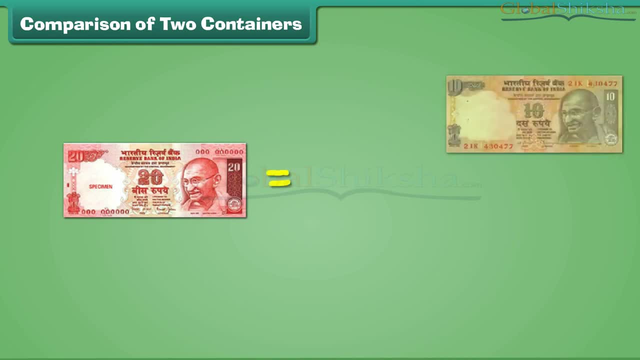 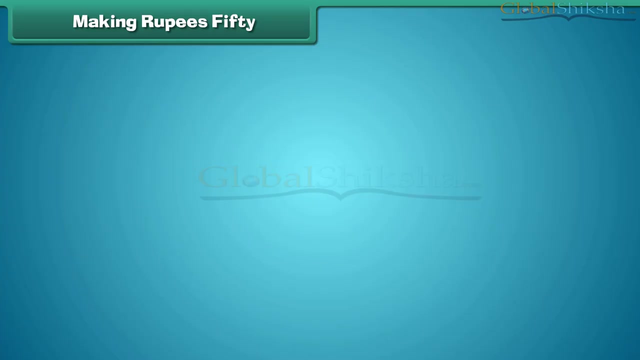 A Rs 20 note is equal to the sum of 2 Rs 10 notes. A Rs 20 note is also equal to the sum of 1 Rs 10 note and 2 Rs 5 notes. Similarly, a Rs 50 note is equal to the sum of. 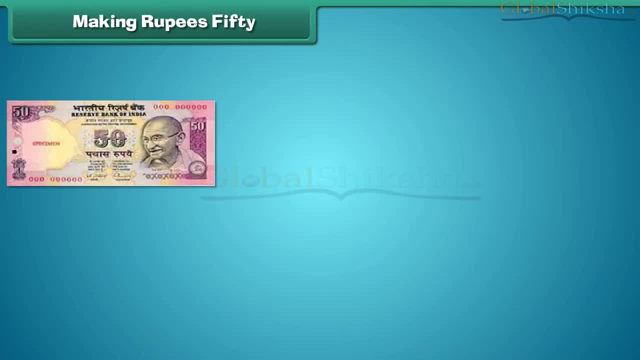 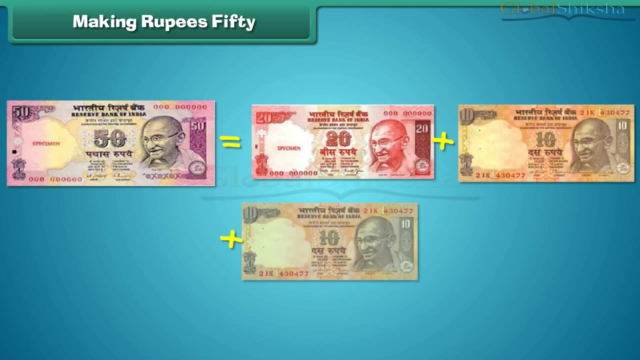 Rs 50 note is equal to the sum of 4 Rs 5 notes. Similarly, a Rs 50 note is equal to the sum of 5 Rs 10 notes. A Rs 50 note is equal to the sum of 1 Rs 20 note and 3 Rs 10 notes. 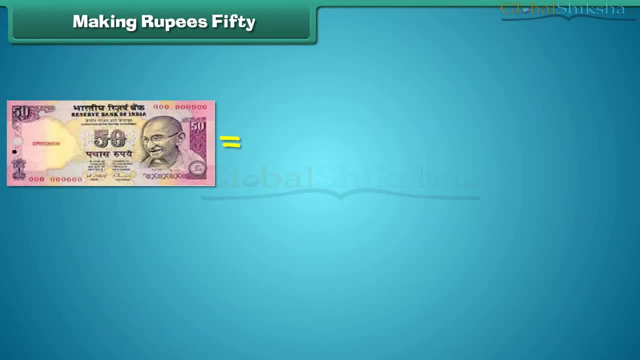 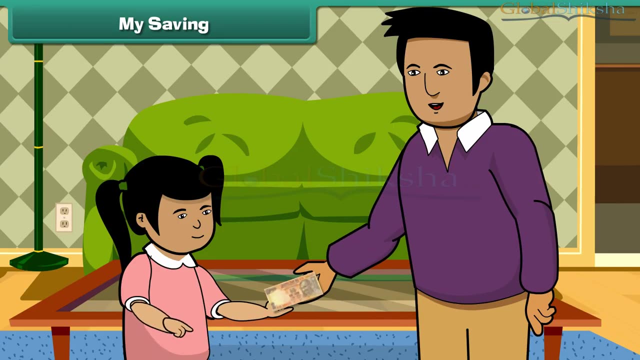 A Rs 50 note is equal to the sum of 2 Rs 20 notes and 1 Rs 10 notes. Remy's father gave her Rs 10.. She spent Rs 2 for buying pencils and the rest she dropped. 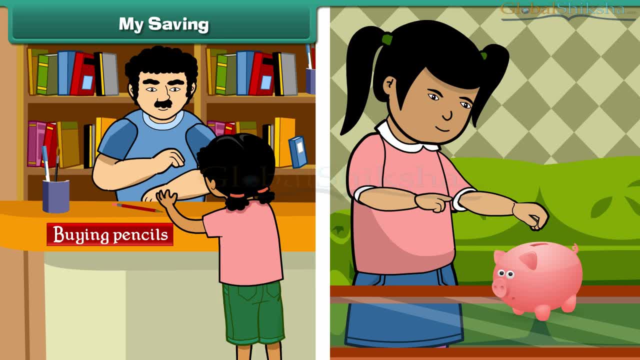 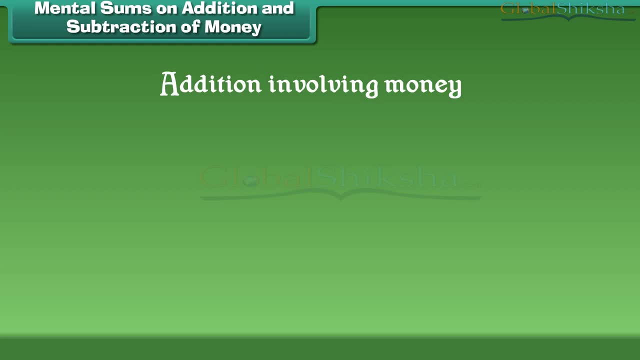 Now let us learn about addition involving money. If I have three 5 Rs coin, then can you tell me the total Rs I had? Add 5 plus 5 plus 5, which is equal to 15 Rs. Now I have 3 50 paise coins and a total of 5 Rs coins. 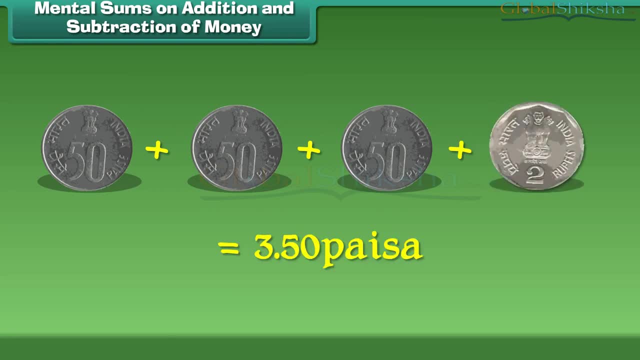 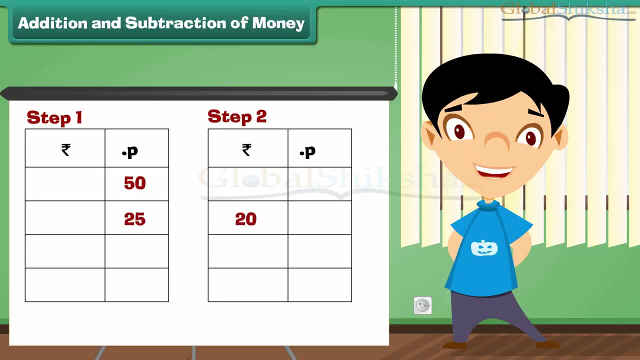 a 2 rupee coin, which is equal to 3 rupee, 50 paise. let us learn how to add 25 rupees, 50 paise and 20 rupees, 25 paise. step 1: add the numbers in paise column. 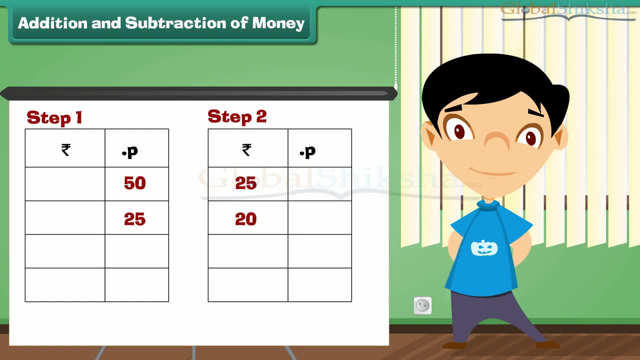 50 plus 25 is equal to 75 paise. write 75 under the paise column. step 2: add the numbers in rupees column. 25 plus 20 is equal to rupees 45. write 45 under the rupees column. let us solve another example. what is the sum of 10 rupees 50? 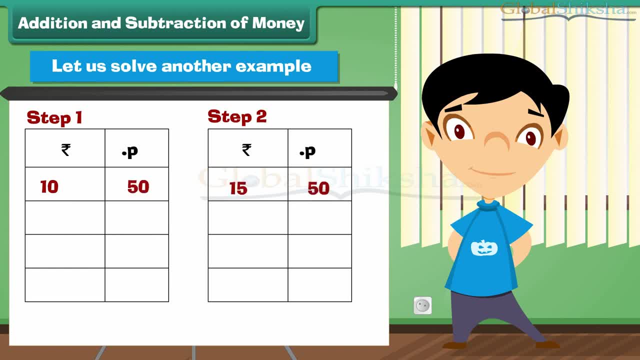 paise and 15 rupees, 50 paise. step 1: write the numbers in correct column. step 2: add the numbers in paise column in paise column 50 plus 50 equals 100 paise. But we know that 100 paise is equal to 1 rupee. 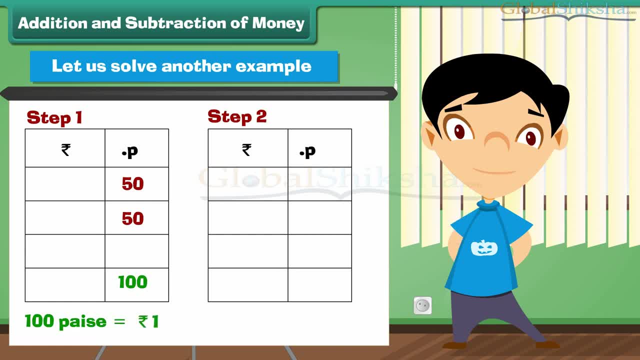 so we write two zeros below the paise column and take 1 as carry. Step 2. Add the numbers in rupees column. 1 plus 10 plus 15 equals rupees 26.. Write 26 under the rupees column. 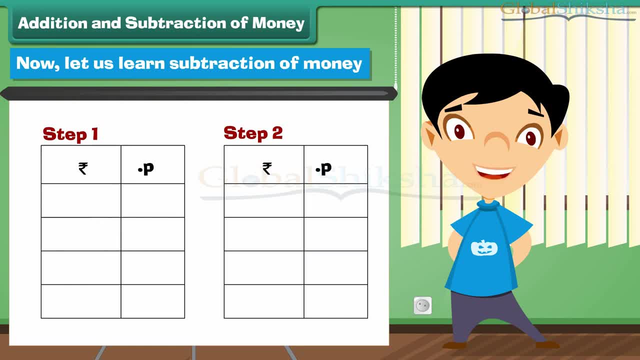 Now let us learn subtraction of money. Subtract 10 rupee, 50 paise from 40 rupees and 75 paise. Step 1. Subtract the numbers in the paise column 75 minus 2.. 25 is equal to 50 paise. Write 50 under paise column.